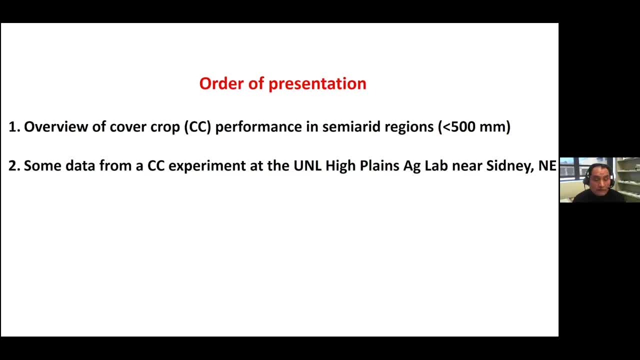 experiment. now is the third year, So Cody Creech, Amanda Sterly and others have been helping us with that experiment at the High Plains Ag Lab near Sydney. But first cover crops in semi-arid regions. I mean, does this make sense? What I would say is: 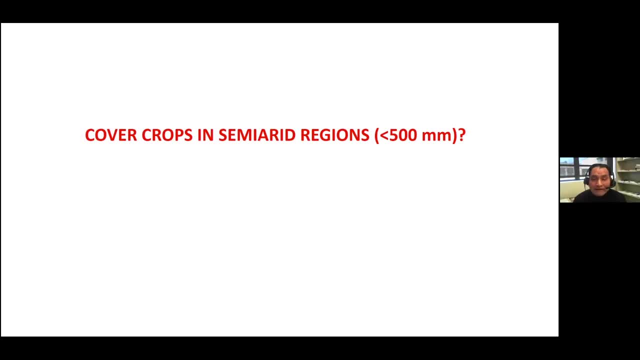 if there is a place on the globe or earth where we need cover crops is semi-arid regions. indeed, I hope most of you would agree with that. I mean in semi-arid regions we have soils with lower organic carbon And some of them are eroded or highly susceptible. 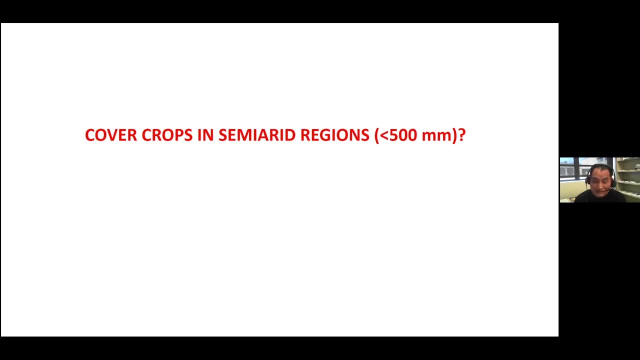 to erosion of what we call degraded soils are more common in semi-arid regions than in high precipitation regions. So why cover crops are not being used by every farmer, right, although the excitement is growing, Right? I mean, we lost a lot of Whiskey crops. We are今日失目に乗る全�� psyche, Okay. 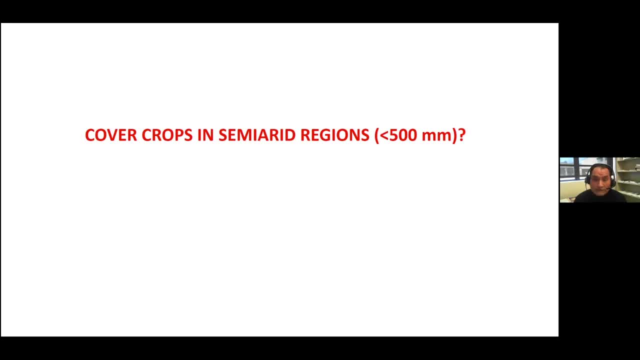 So why is it so bad now that each sober crops are not being used by farmers, right? Although carbon from the regions like other regions, right, that's something about 50 percent of carbon is gone. i mean, jay showed you know differences in organic carbon or organic. 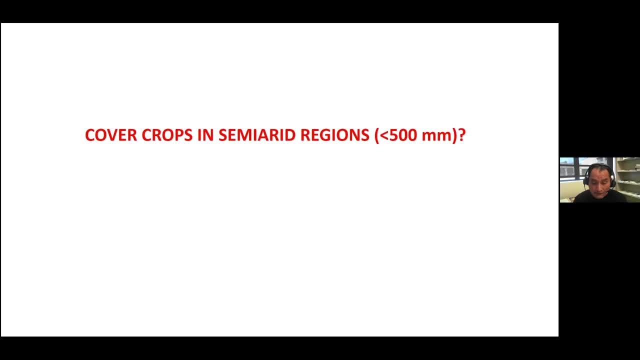 matter among different management practices, right, so it clearly shows that, yes, by managing the soils intensively or telling we lost a lot of carbon, now then we need some medicine. then, right, you guys discussed earlier, i mean this: healthy soils may not need to see the doctor, but soils that are degraded need to see the doctor and one of the pills that can be prescribed 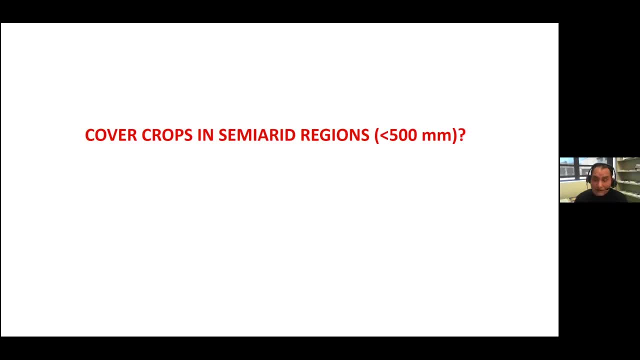 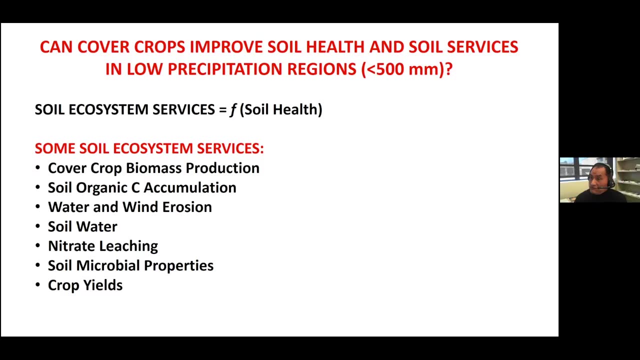 is cover crops, right. so how come cover crops are not being used to earn spots where they are needed the most? so i'm gonna touch a bit on this. and okay, i've been asked to talk about soil health. uh, but bijesh and others, um, but i'm gonna link uh soil health. i mean, i know jay defines well health. 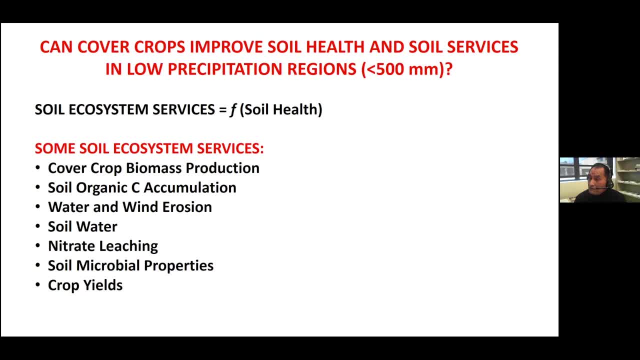 greatly. if the soil is healthy, uh can deliver many services right. i mean a function properly. so i'm going to talk about ecosystem services that we get from soils. i mean, if we have a self, this healthy system, a healthy soil, i think we can produce a lot of biomass right, or probably accumulate a lot of. 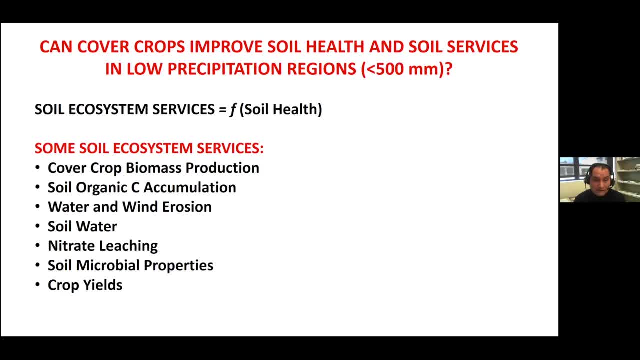 toru, see altogether soil and have about like arian or even so. now, today, especially as a lot talk about carbon sequestration, now, carbon credits, right, can reduce water and wind erosion, right the soil water can be. obviously, you know, cover crops use water, but what about the residues? uh, what about leaching? 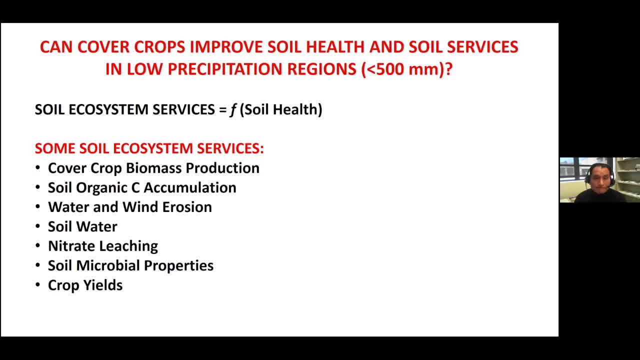 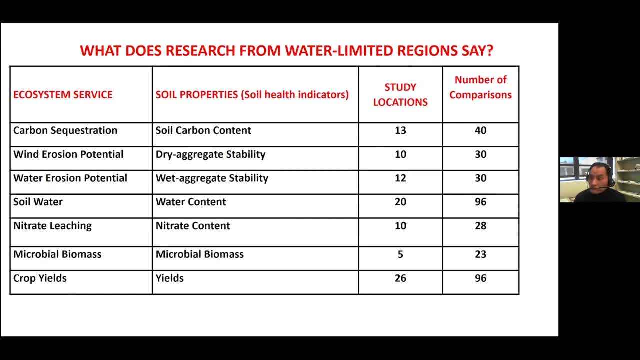 so i'm going to link um cover crops to these services that we get from yields and obviously crop yields right. what i've done in the past few um amount is a summary of what we knew from research data conducted in similar regions. that includes arid, and similar regions are less getting less than 500 millimeters of precipitation. 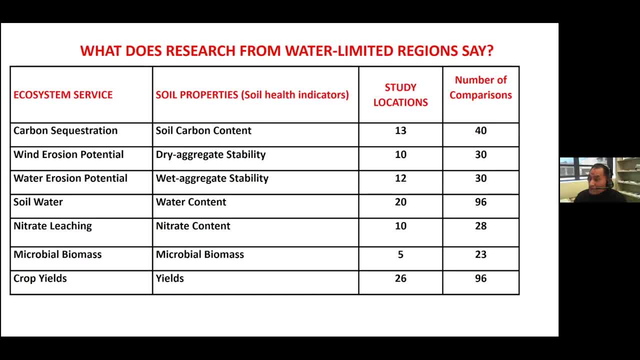 okay, so here we have some soil health indicators properties. there are 13 locations. what about erosion? i mean, they have not measured specifically actual wind erosion or dust blowing, but it's more about, like you know, dry aggregates, the weather, weather aggregates, the measured water content, nitrate leaching on their cover, crops and right. and then i looked at the comparisons. there are a. 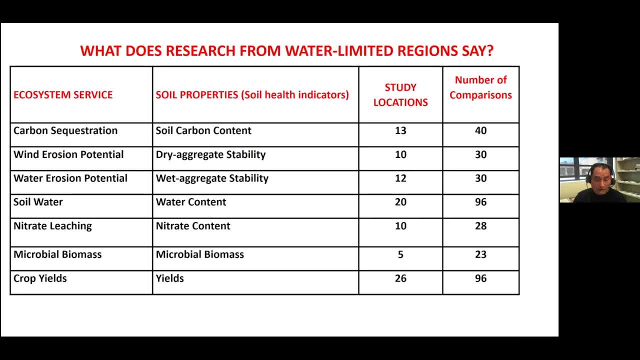 good number of comparisons there, so we have data. this is mostly data from the us great plains, so that includes uh, northern central um and southern great plains and all. we also included a few studies from other parts of the world. i mean like in, you know, in spain, i mean in southern spain. i mean we have 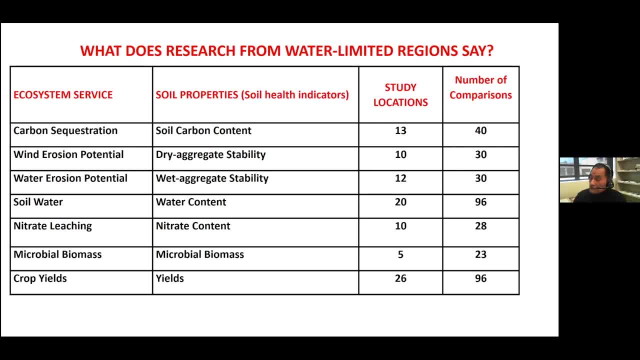 some samaritan soils and another regions, but most of the data are from the us great plains. i think we have good number of studies, especially with comparisons. i mean one study, let's say that they have compared. you know control again against, you know several cover crop species. so the comparisons, well, will be a large number. 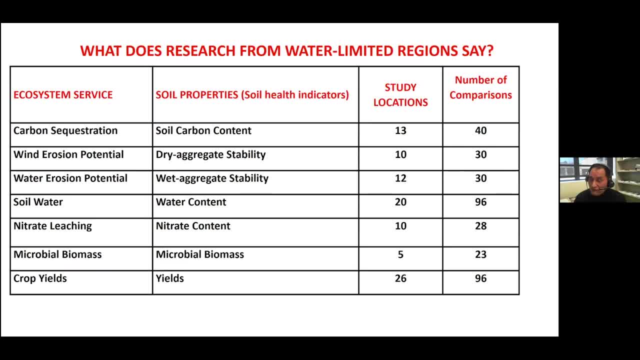 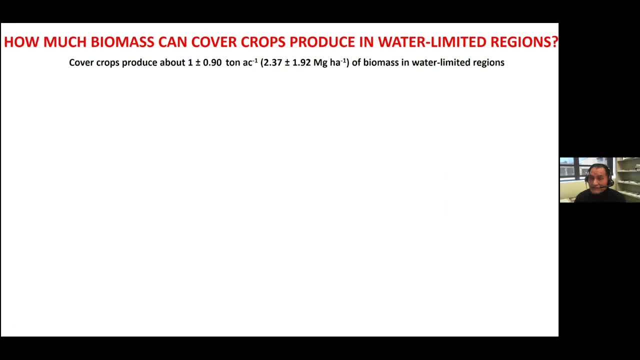 and within the same study. so what do we learn then? can cover crops produce biomass and water limited regions. these crops use a lot of water. here is an average number, okay in english units, so you can see that the average number of crops that we get is about 1 ton per acre. 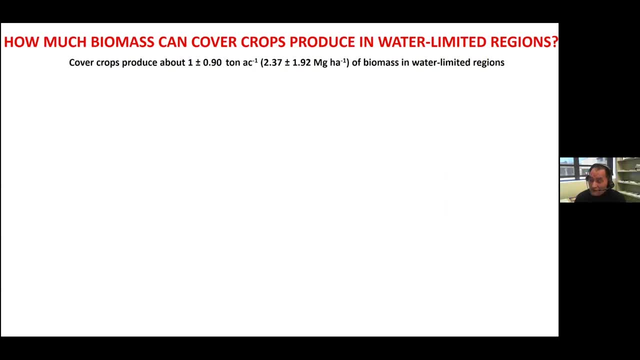 and the average number of crops that we get is about 0.9 tons per acre. wow, look at that standard deviation. but yes, one ton is not that bad, it's an average number. it depends where you are or where you are farming, but this average is promising. it is a bit lower than what we get in high precipitation. 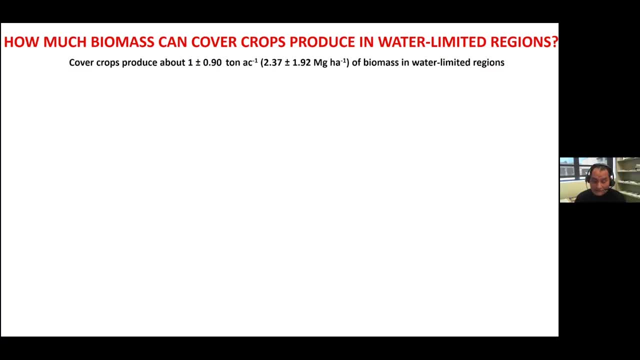 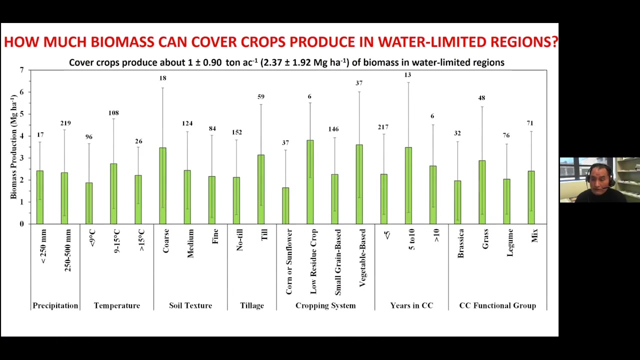 regions, but it is, it is significant the above ground biomass production. what about root biomass? let's not forget about that portion, right? so i'm gonna cover that later. but there is high variability, obviously. i mean, we can spend here, they can spend the whole day talking about this, right? well, you said less than 500 millimeters. 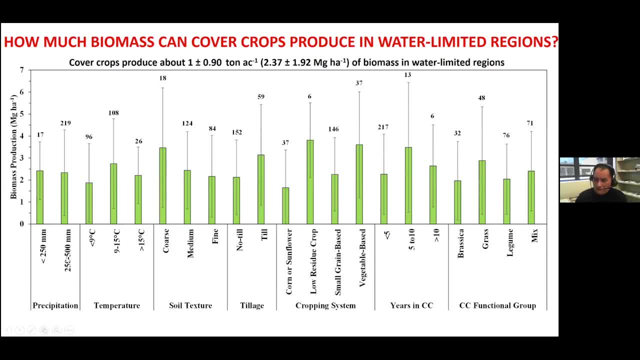 well, what about then? we have some studies in that summer. you know, looked at, you know, even in less than 250. what are these regions? i mean california, i think in a couple of spots there. i mean these are a number of comparisons we have here biomass production, right, and then our biomass production, and then it's yeah. 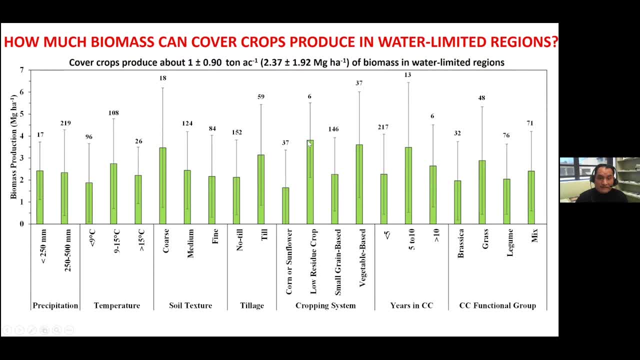 look at that. in some cases this is in metric units, obviously, and then this is about what? four, and it could be about two tons, right, right, yeah, but in some cases it's just not much. so then, average. we are getting this much on the different regions, so high variability. 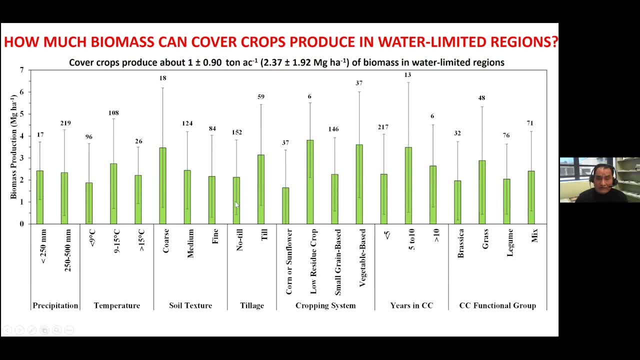 probably depending on on the system. i mean one thing here. look at this and that i was surprised when i saw this: no till, what about putting cover crops after no till or after tillage? look at that. it seems that i mean this standard deviation is high, but it seems tillage does not matter much. 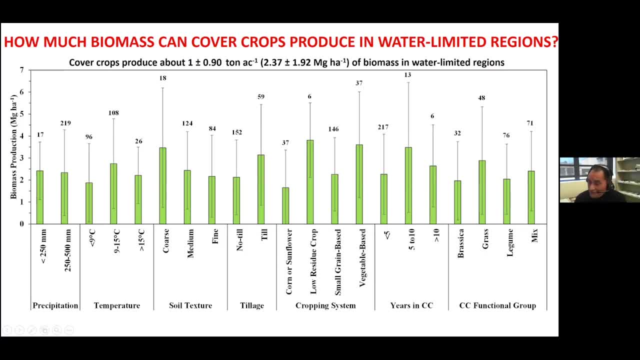 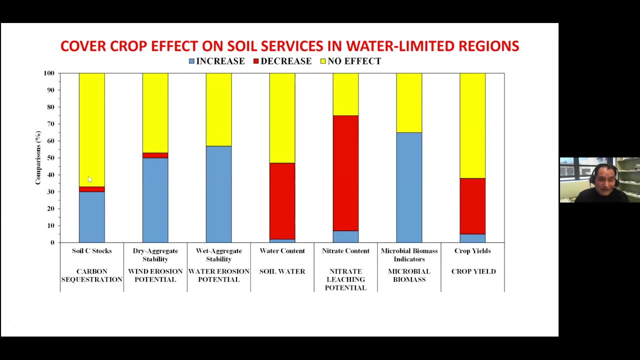 interesting. this is a summary that the studies in semi-arid regions- or that includes arid regions- can cover- crops sequester carbon in these regions. well, well, this- I was surprised about this a bit. not really. it can sequester in about 30 percent of soils, so it seems in most cases we're not sequestering. 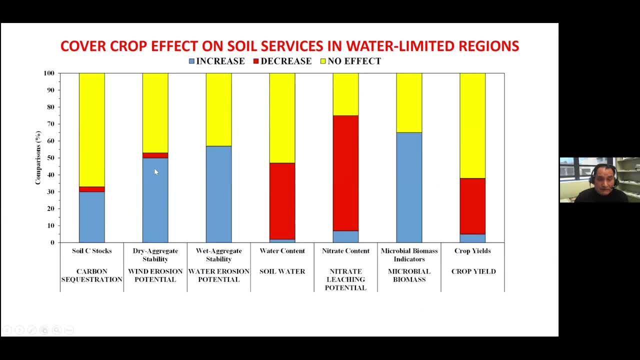 a lot of carbon with the cover crops in this region. what about, uh, this? what we're reducing, when the fraction was that related to dry aggregate stability? yeah, the blue and stems: we are increasing that size of aggregates. the same thing with the water erosion: we're increasing the size of aggregates. that's a good thing. what about? 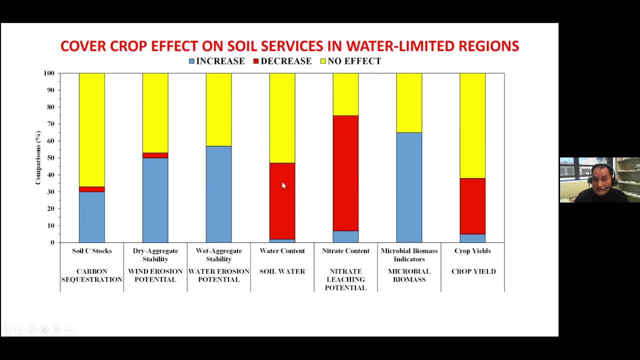 water, kind of 50- 50 here. it seems that no effect in half girl, right. and then it reduces in up maybe about 40 percent, right? what about leaching? we've been using a little bit too much nitrogen in some cases and then can cover crops reduce leaching. yes, look at that it's about maybe. 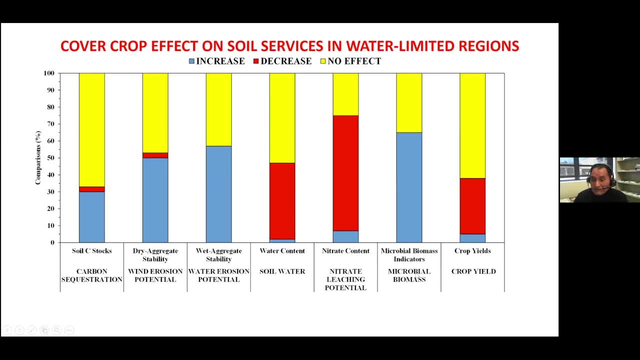 60 percent or so. what about biology? well, that's one of the parameters that we look at when we talk about soil health, right? yes, in most cases, about 60 percent of cases. yeah, adding cover crops- and you know, soils and semi-arid regions can increase microbial biomass, for example. what 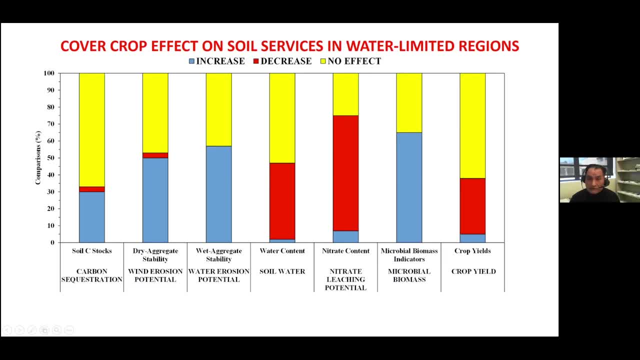 about yield. at the end of the day, that's probably some people care. most interesting that in most cases it seems cover crops do not really reduce yields. but i would say maybe one third of cases, 30 percent of cases, yes, you can reduce. what's the message from all this? is that it cover crop. 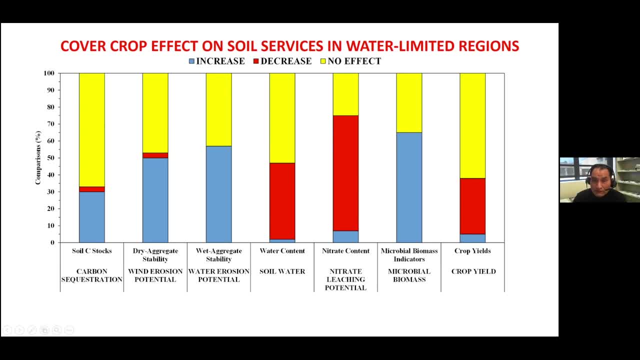 performance or effect on soil, health or ecosystem services is highly context specific. so if a farmer is seeing a lot of benefits on his or her farm, the neighbor boring farmer may not see that, may not see the benefits. and we can touch about the factors for that divergence a bit later. 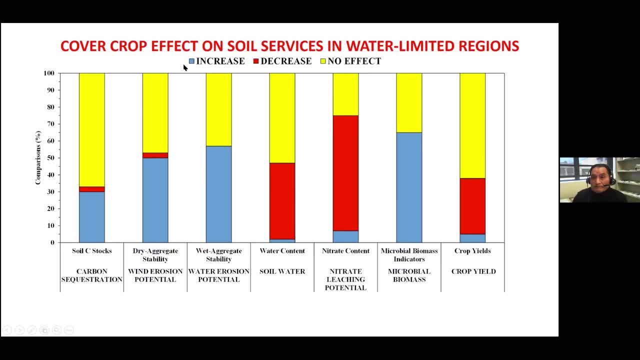 So how do cover crops? you know change with climate, soil management, for example, Interesting in terms of, you know, the carbon content here. This is the carbon content differences. I'm not going to. I can spend again a lot of time on here, but we don't have a lot of. 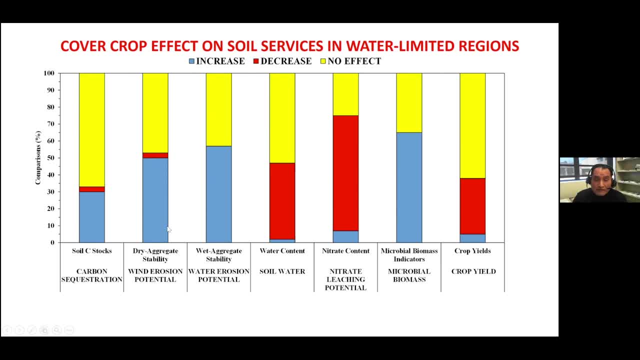 data from coarse, from sandy soils here. So a couple of just points from this graph. Look at this: no-till against no-till. Well, no effect, it seems, in both systems, right, Obviously? I mean, we don't have the same percentage of comparisons, right? 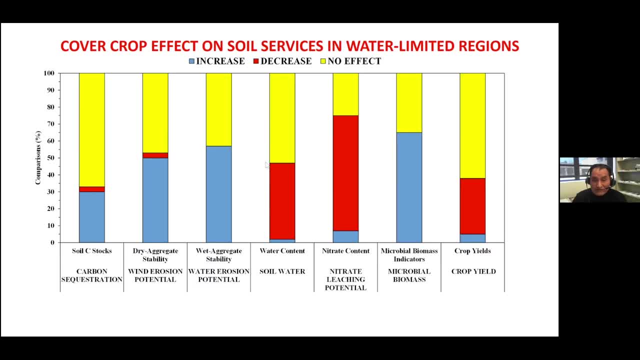 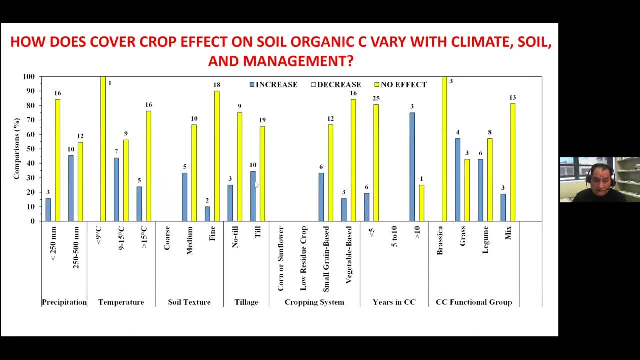 I mean this is not, This is nine. I mean it seems most of the studies in cover crops and similar regions have been conducted in tilled systems. but in short, nothing much there, no differences due to tillage. And then about this is sad. I mean not sad, but this is actually a fertile ground for 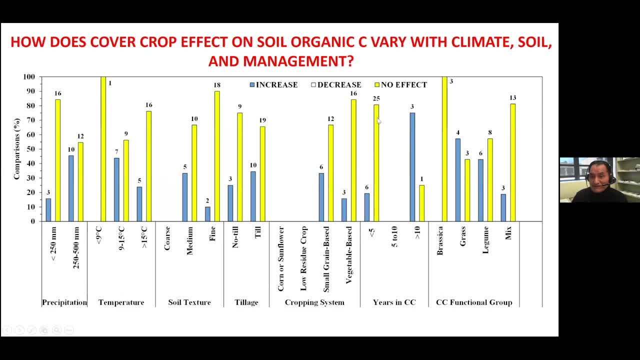 us for researchers. We have a lot of short-term studies. We don't have that many, only one there. this is in terms of comparisons, right? So not many there, Right? So what about mixes, Something that people talk about? 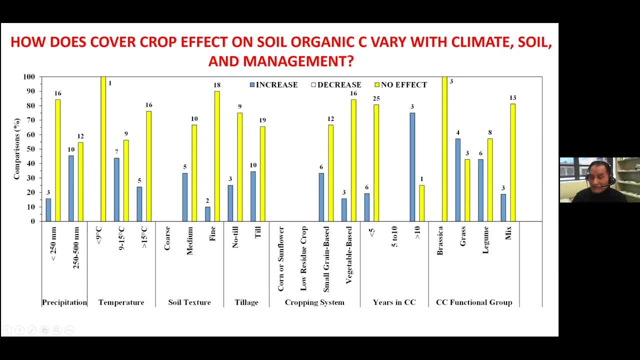 Oh, let's put some cover. crop mixes, cocktails will do better than single species. Well, not really, not really, but increased, I mean it seems actually a little lower here. the tendency, right, I mean it's grass, yeah, like rye triticale can do better than mixes. 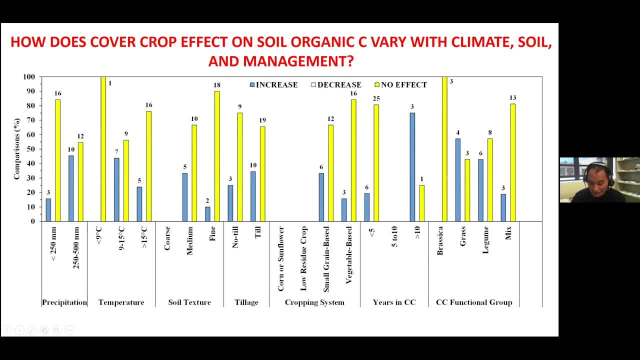 I mean, that's another topic, but in short, it seems that mixes are no better than single species. What about microbial biomass? Right, This is microbial biomass. changes related to soil health- right The same thing. A couple of points here. 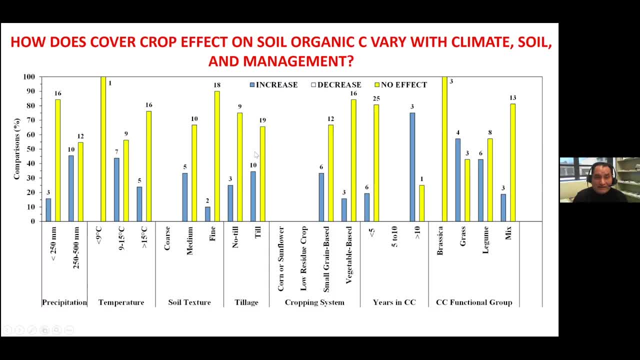 From tillage, it seems that it doesn't really matter. Indeed, under tillage systems, cover crops can increase, probably tend to increase more, you know, microbial biomass- than under no-till conditions, but it's some variability there. but again, that is not. we're not increasing, more probably improving soil biology under 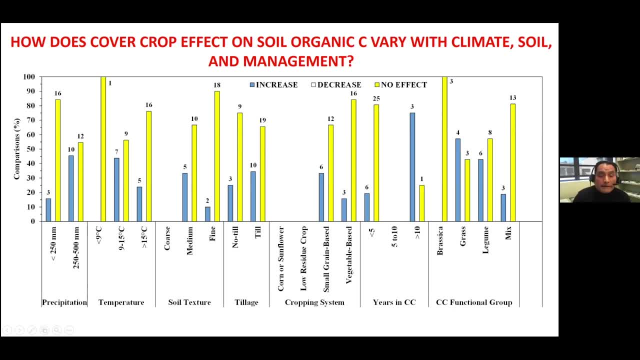 microbial biomass Under, you know, no-till cover crops- I mean under cover crops- are not doing better job under no-till than till conditions. that's what I'm trying to say. What about mixes? Again, no advantage for mixes when it comes to improving soil biology, because performance. 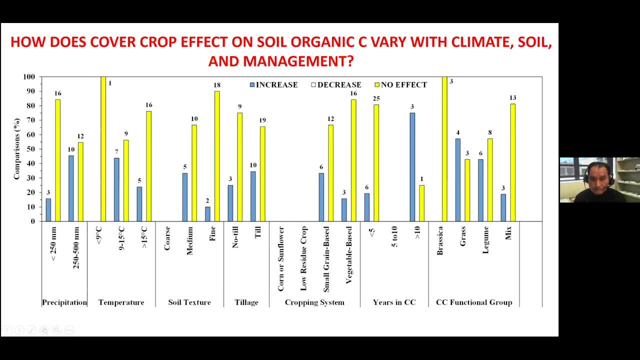 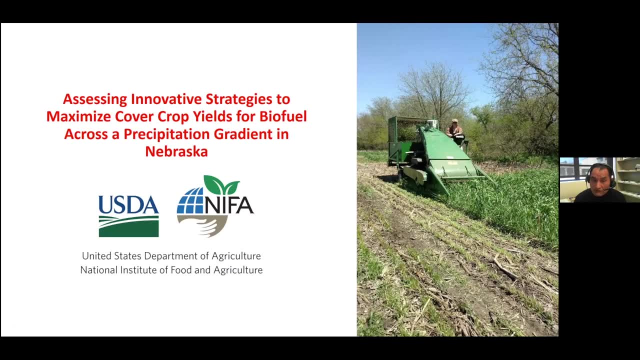 is similar to single species. Okay, So that's an overview. That was an overview. So what we know so far from research conducted in arid and semi-arid regions. I mean, I can go back and this is probably again the summary of what we know. 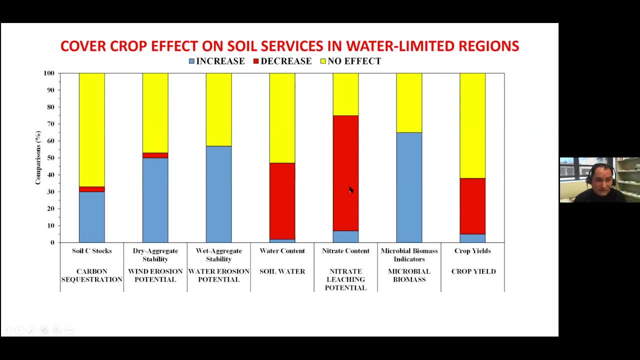 I see a lot of benefits there. Like in carbon, it may be questionable: well, this is not well. your farm may be here or may be here, right, So it's highly site-specific, but definitely we are reducing erosion potential. 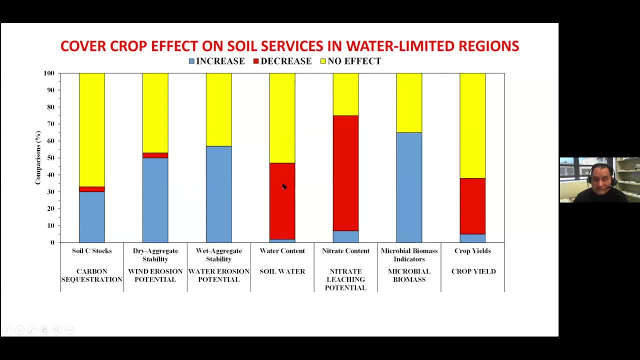 Well water. I mean, yeah, we're reducing in some cases. What about leaching? I mean, cover crops can provide benefits and we're definitely. we're improving microbial biomass and, in terms of yields, no effects in most cases, it seems. 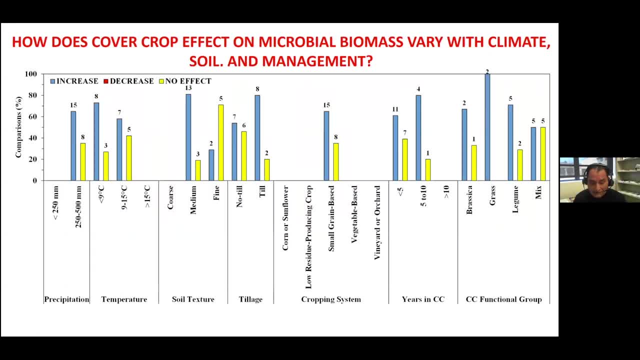 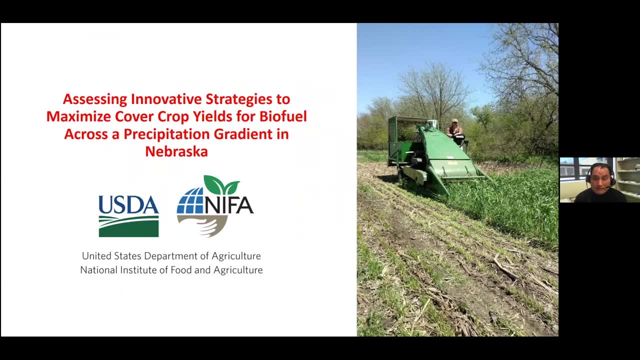 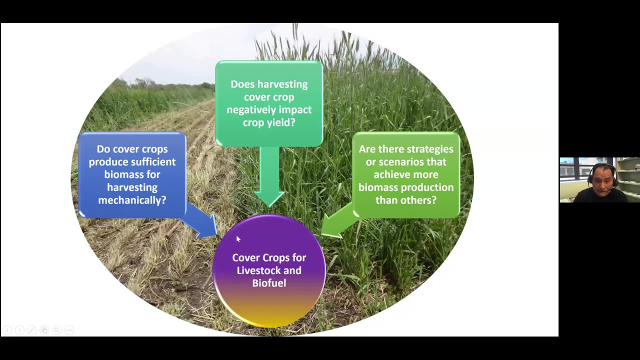 Okay, Now I'm going to share data from the High Plains Ag Lab experiment. This project is funded by NIF, So it includes harvesting cover crops could be for biofuel or for livestock haying right. So these are the questions that this regional project is addressing. 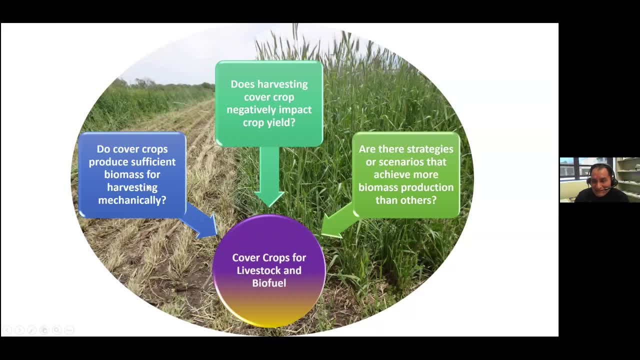 Do cover crops, produce enough biomass for harvesting? I mean, in some cases we cannot even establish Okay Or grow, you know, get enough biomass to improve, you know soil properties or health right. I mean, now, on top of that, you're going to harvest. 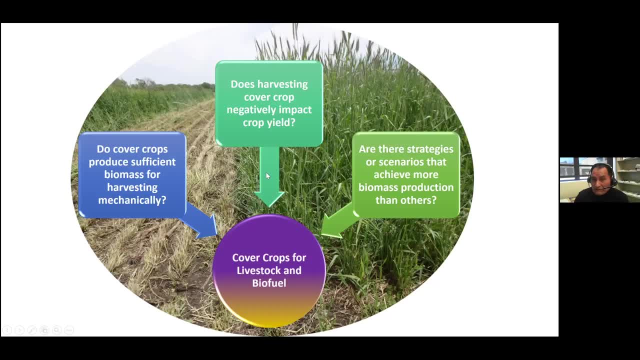 And then does harvesting cover crop affect crop yields? Well, we have seen that cover crops, you know, growing cover crops can reduce yields in some cases. but what about harvesting? Are there strategies that we can use to increase biomass production in, you know, in different 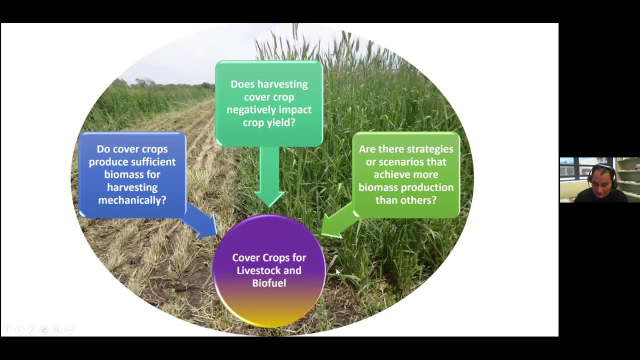 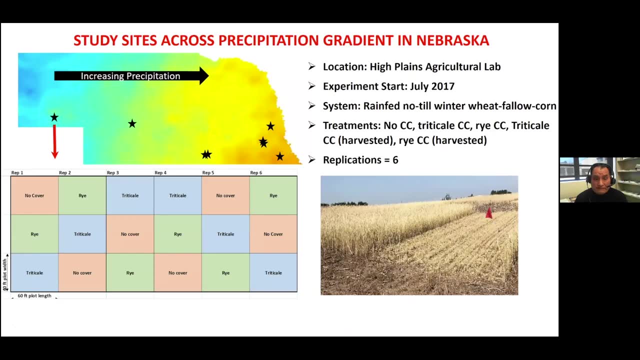 regions, right. So this would be an interesting right. I mean, we can get some benefits from economic benefits from cover crops, right. So we have a good number of studies across Nebraska, And then I'm going to talk about specifically this one. 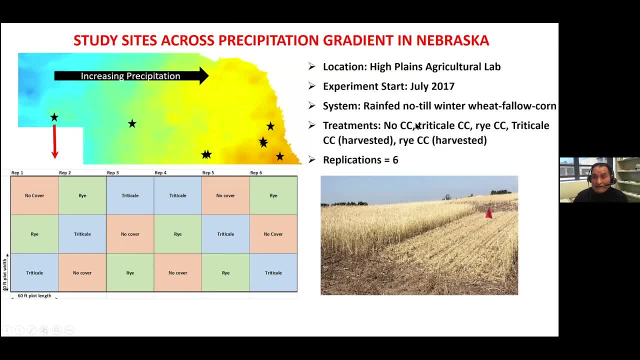 This is a randomized complete block design have near High Plains Ag Lab started in July 2007.. Rainfed: no till winter wheat. fallow corn Treatments: no cover crop. Critical cover crop. Rye Triticale harvested. 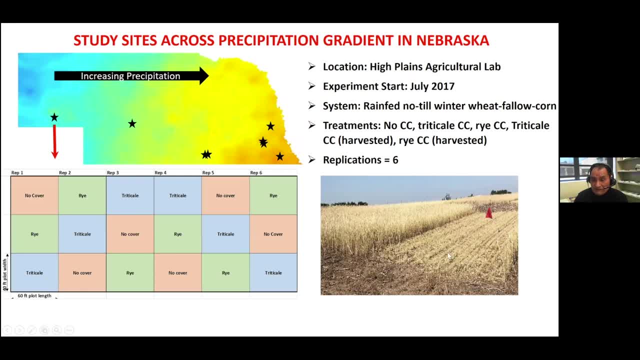 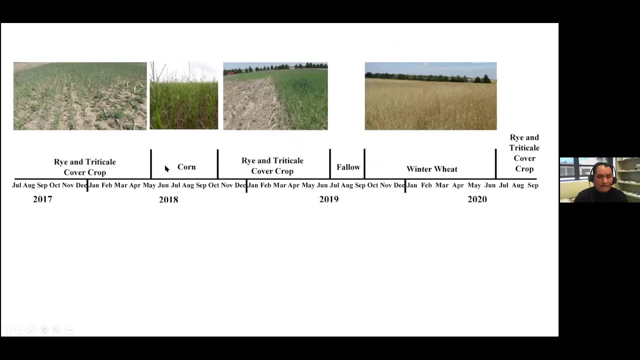 Rye harvested Replication six, So that's four of in one year where we harvested cover crops for Cody Creek. Okay, So this is it? just what system? So this is the wheat with the fallow corn. So we had the rye and triticale cover crop planted in July in 2017, then the following: 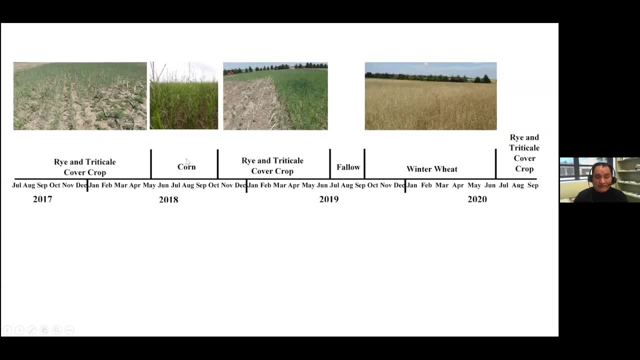 year, in 2018, it was terminated around May, Then we planted corn, Then in October we planted rye triticale and then we killed that mid-June or so. then this was fallow, Then winter was winter, wheat was planted. 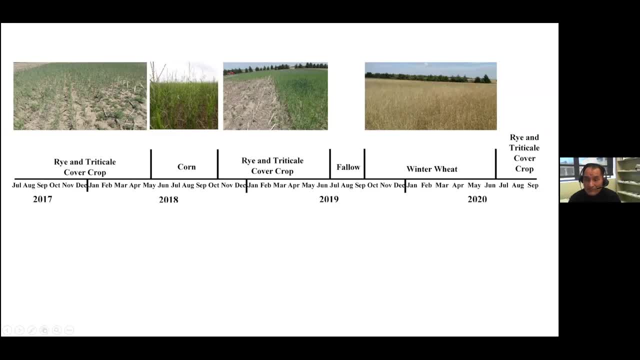 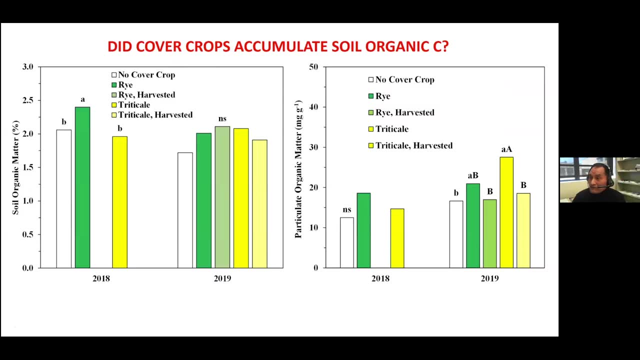 And then right now we have rye and triticale growing there, hopefully. So, okay, What do we know? What did we learn from this? the cover crops accumulate soil carbon. So it's the data on carbon. This is after one year and this is after two years. okay. 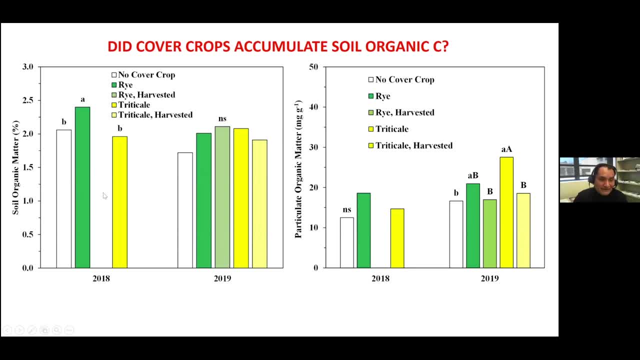 So after one year? after one year, organic matter it increased slightly from 2.1 to 2.5, interesting with dry but not with criticality. What about after two years? This high variability? a lot of times this happens. 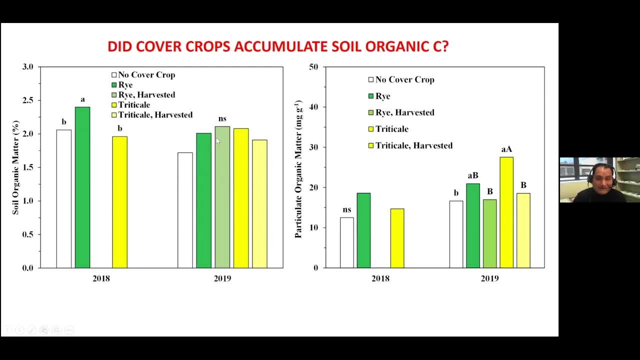 we have observed. that's why we need long-term data In second year. yeah, there was a tendency, but it seems that there are no significant differences there. What about the live vial fraction? I mean, we need a lot of times. 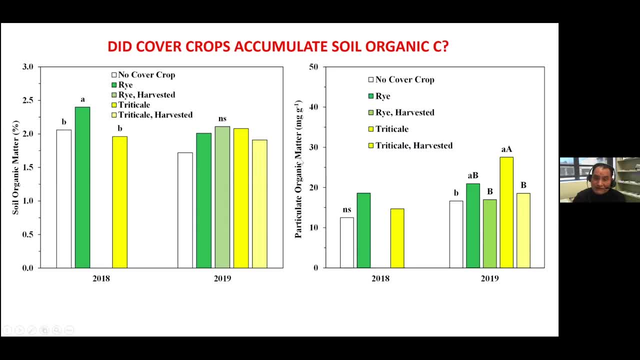 that live vial fraction changes more with management. So the particulate organic matter: we didn't see anything in the first year. As I mentioned earlier, we had harvest component as well. Obviously we didn't have. we didn't impose the harvesting treatments here in 2018 yet 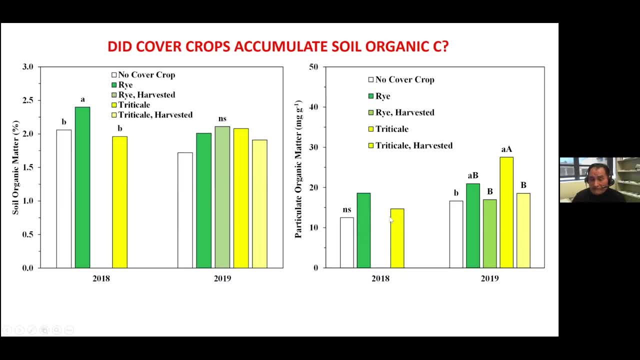 before sampling, then we imposed after soil sampling. So then, yeah, nothing in terms of particulate organic matter differences. What about after two years? We have an increase. we see an increase in what we call POM, with dry and then with criticality. 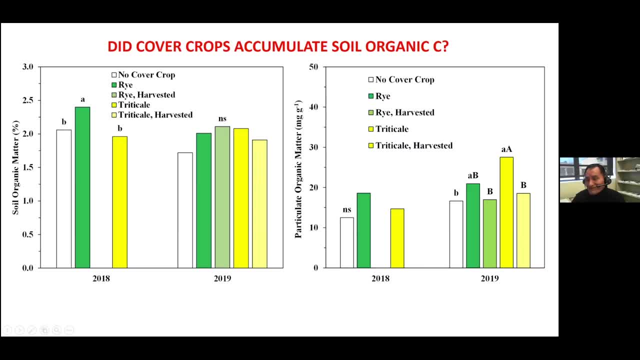 but it seems that harvesting kind of tend to reduce that benefit Interesting trend here, right. So I mean harvesting, it seems, but it's not worse than not having cover crops, I mean, but it seems that it reduced the benefit when it comes to POM. 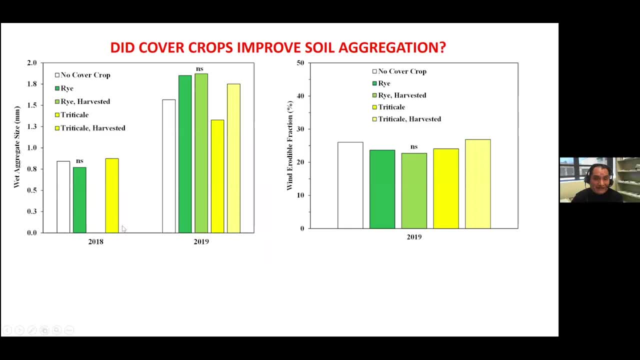 What about soil aggregation? Soil aggregation, So this is a wet aggregate stability. you know, wet aggregate size: nothing on the first year, nothing on the second year. Some variability there, but it seems here, in this case it increased a bit. 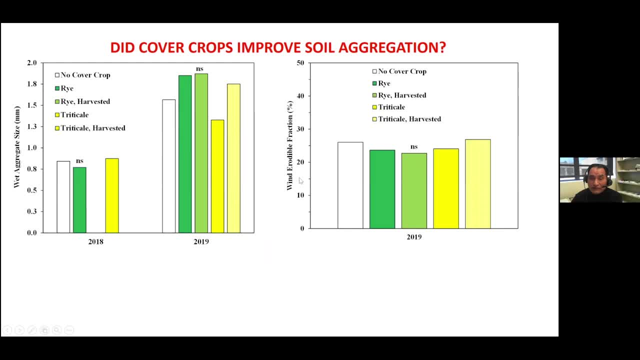 but here it decreased. obviously it's high variability there. What about the wind-redeveloped fraction? That's what was related to this. It was related to dry aggregate stability, the dry aggregate size. Obviously, the more you know, the larger this number is. you know, the worse, right. 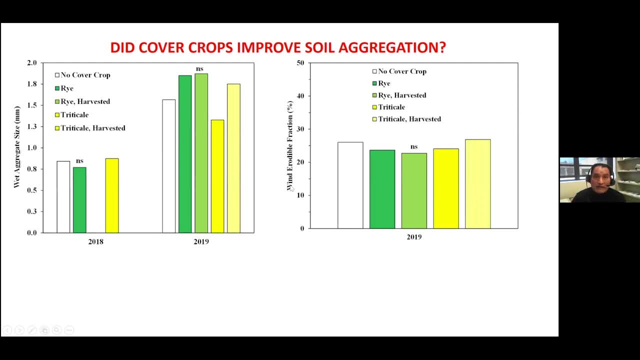 Because, as it refers to the smaller particles, So here, well, obviously, control tends to be high, right, But then when we add cover, crops tend to lower. that that's good thing. But again, there is no significant difference There, right? 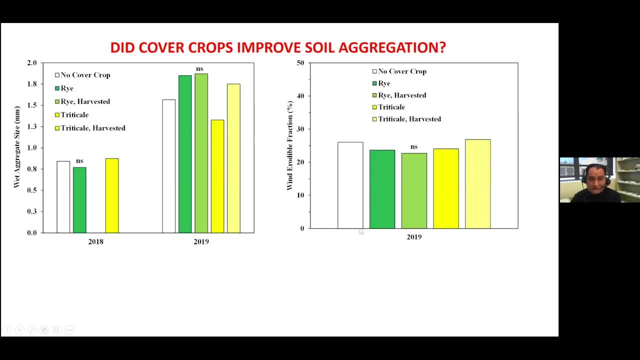 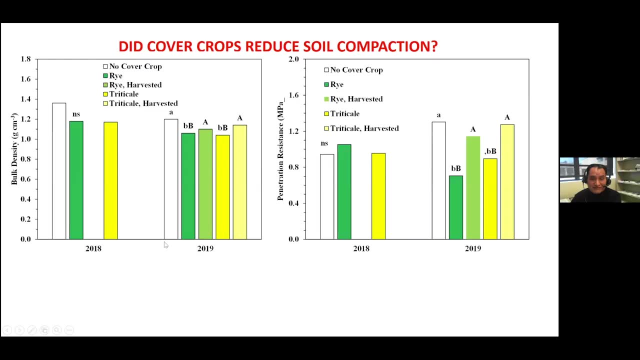 But there are some trends, So we're going to keep monitoring this in the coming years. What about compaction? This is something we don't hear about. special and semi-arid regions, Oh no, that's not the main, you know. 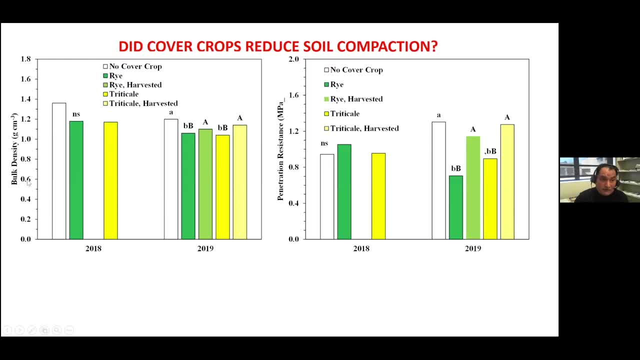 it's not the hot topic probably, but we did measure compaction as well. Bulk density, penetration, resistance, Those are the parameters, right? Nothing on bulk density in the first year. What about in the second year? Well, there was a decrease there. 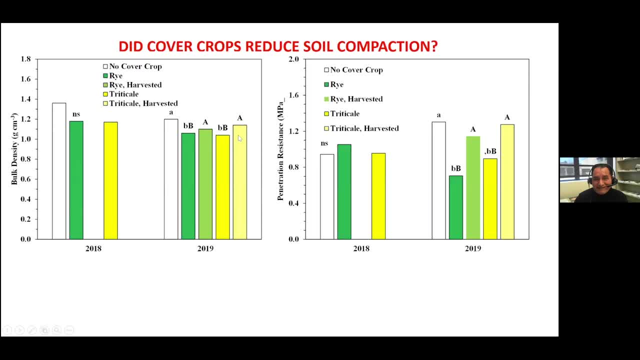 Right, But it seems harvesting tended to increase. that This is an interesting data. I mean, I was just short term data, but okay, bulk density yeah, increased with cover crops, but then harvesting probably due to machine traffic, right. 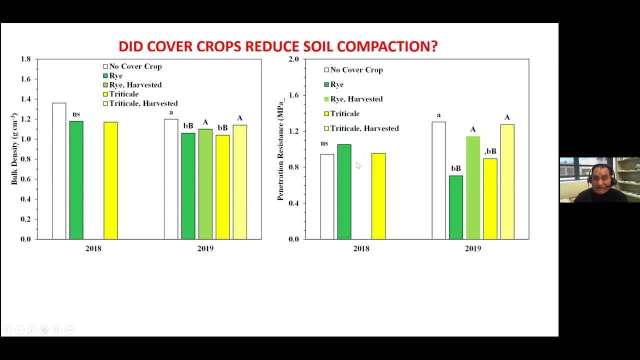 It seems that tended to increase that. What about penetration resistance? Nothing on the first year and the second year, Yeah, again similar to bulk density. it seemed to reduce penetration resistance. right, And both are right and critical, but harvesting tended to increase, you know. 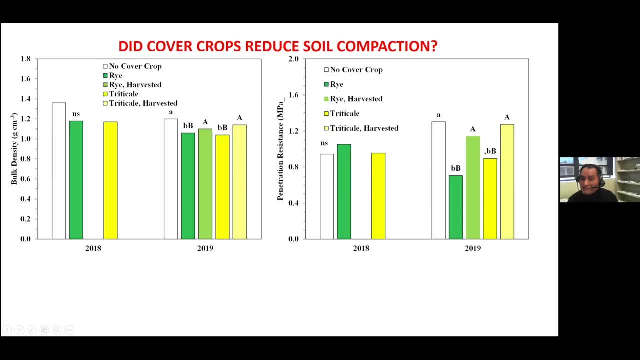 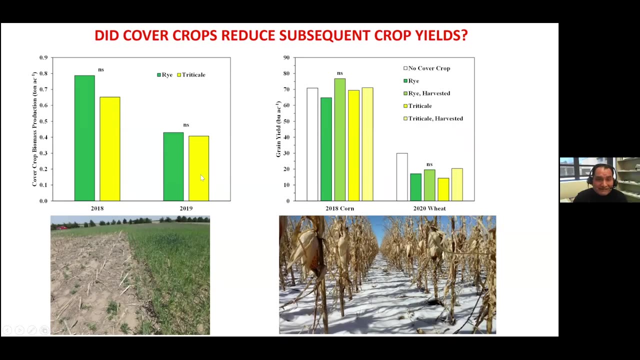 the compaction tended to eliminate the benefits of cover crops. It's again machine traffic, right? So important to remember that you know, obviously traffic can cause compaction. What about yields? Tell me about yields, Okay, so here we go. 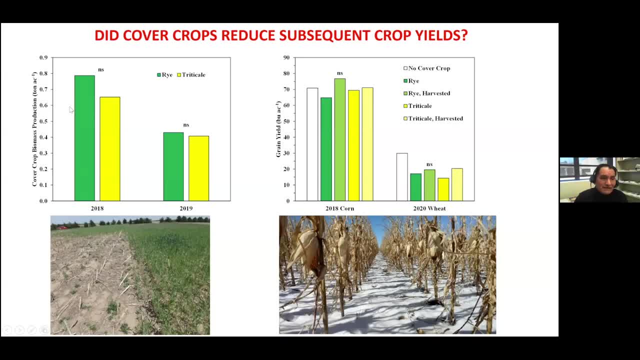 Here is a cover: crop biomass production in first year in tons per acre. Okay, 0.8, 0.65 in the second year. Yeah, depends on the year. Again, look at that about 0.4 in the second year, not much. 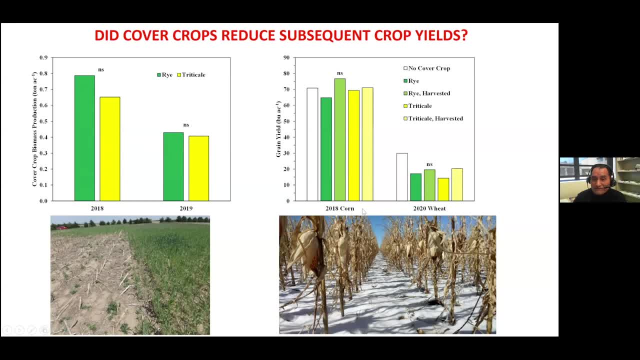 Right, And what about yields? Corn the first time, and then wheat. Some decrease nothing, non-significant differences Here. overall there's a decrease, but again with you know 5% level of probability and statistics. researchers talk a lot about that. 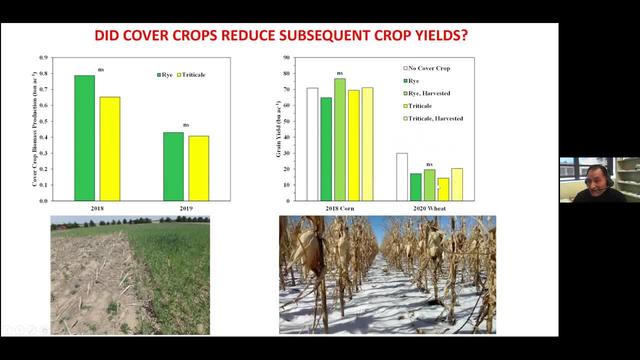 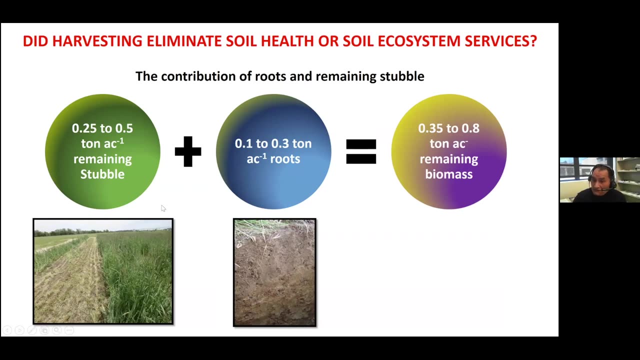 I mean in terms of bushels per acre. there is some decline there, but there is a high variability again. So some decline, but not statistically significant. Okay. So what about harvesting? It seems like an organic. I mean did not really reduce organic matter content. 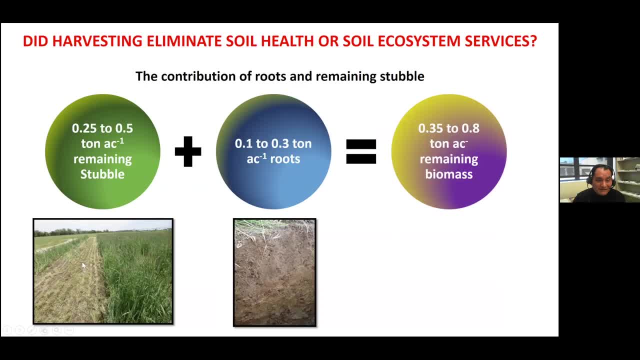 the particulate organic matter right. So if we are, you know, harvesting like this and we are not harvesting the roots, so I think there is still some benefits from that right. I mean, this is the remaining stubble after harvesting. 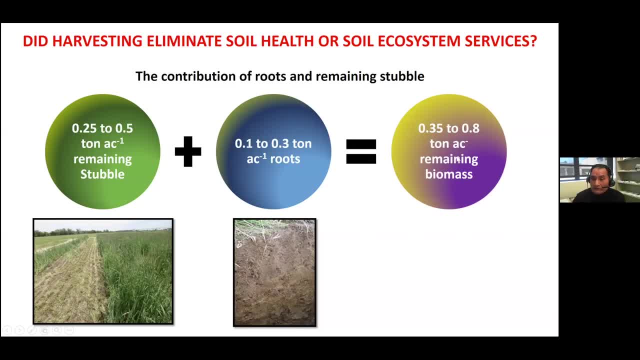 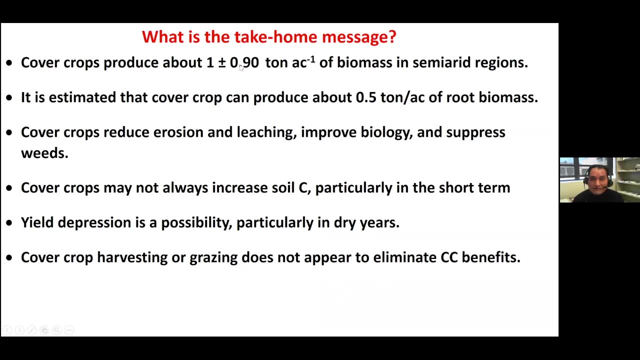 then we have roots remaining and then the total biomass remaining after harvest. I mean it's not that bad. It's still significant that enough to maintain cover crop benefits. So what's the take-home message from this? We mentioned about that, the amount of biomass produced. 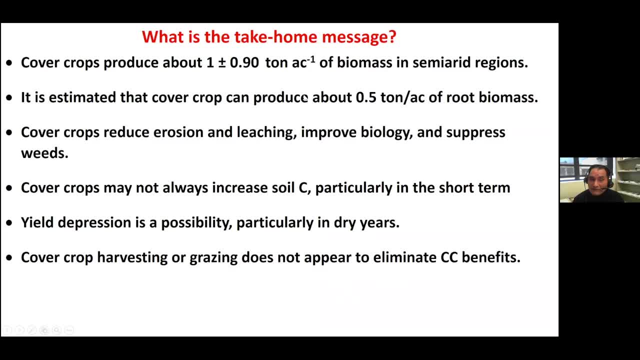 but let's not forget about the root biomass. So what's the take-home message from this? We mentioned about that- the amount of biomass produced, but let's not forget about the root biomass. we don't have a lot of data. It's something that we are getting busy now. 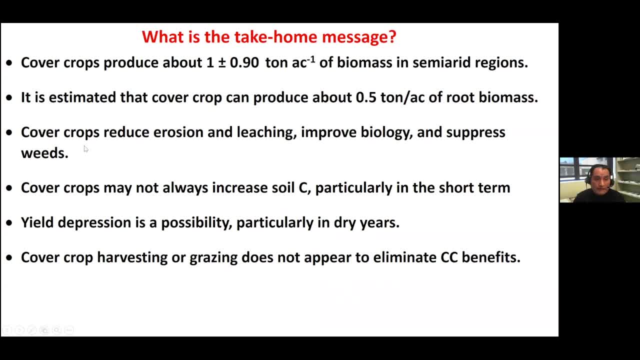 We really need to look at the below ground portion, And we know that, yeah, cover crops reduce erosion, leaching biology, and then wheat, something that I forgot to you know to discuss in depth. It's not in my field, I'm a soils guy. 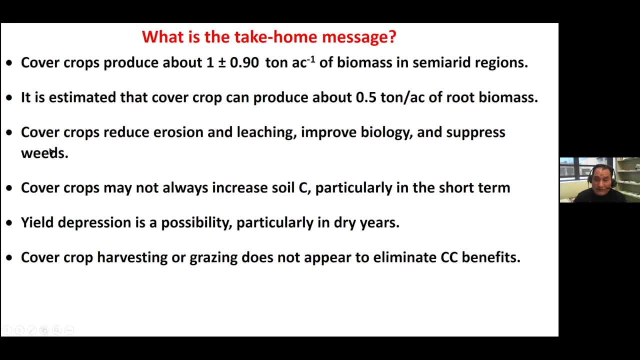 but yeah, I've seen cases where, yeah, in some of my plots- I mean when you have cover crops, you don't see any weeds, but then the neighboring plot, what we call control- without cover crops, we see a lot of weeds. 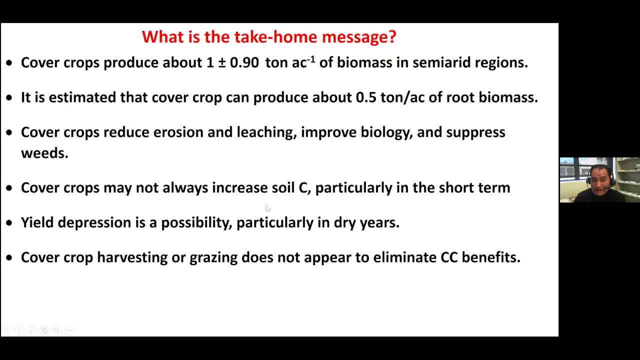 So important to remember that cover crop might not always increase soil carbon, particularly in the short term. Well, yield decrease yes, it can happen, especially in dry years. So harvesting or grazing, I mean I don't think it will reduce the benefits of cover crops. 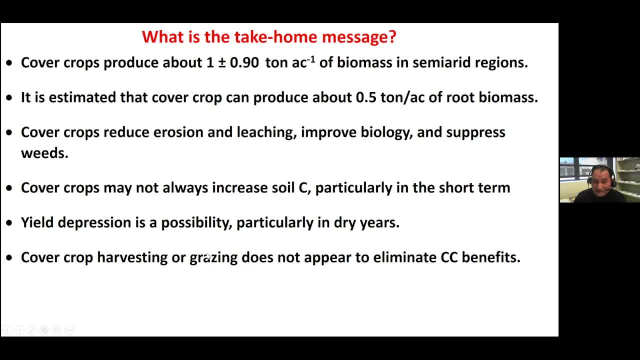 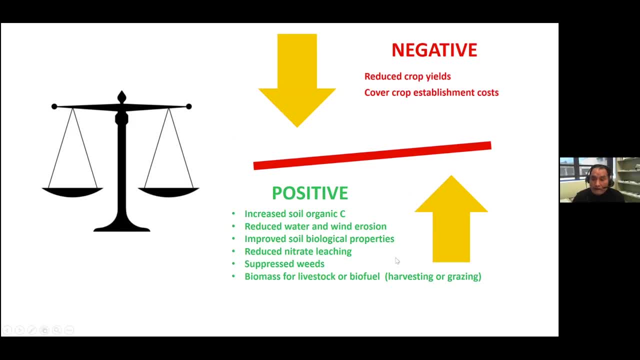 It's not going to be worse than control, And now you can get some economic benefits from there. right. Couple more slides here. OK, I think we have negative aspects when it comes to cover crop adoption, right. Obviously, a negative aspect is: 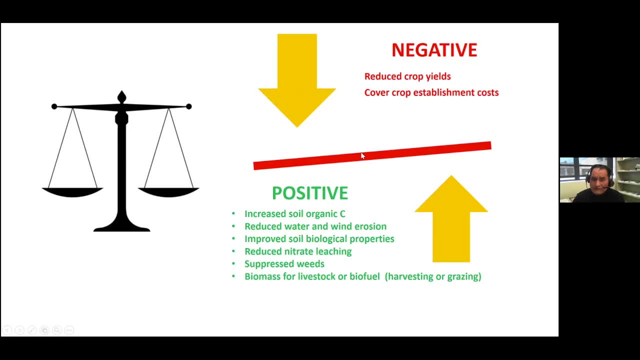 that we can reduce yields in some cases. And what about the cost for cover crop establishment? I think we need to balance that right with positive aspects: An increased organic carbon content in some fields, specially if we- you know, if we get to this. 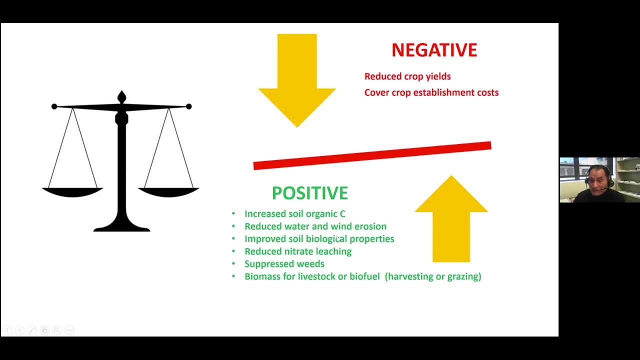 let's call the carbon credits right- Not about water and wind erosion, biology or soil health were improving. What about reducing leaching? What about weeds? And this at the bottom right? We have a good number of experiments with this as well, and 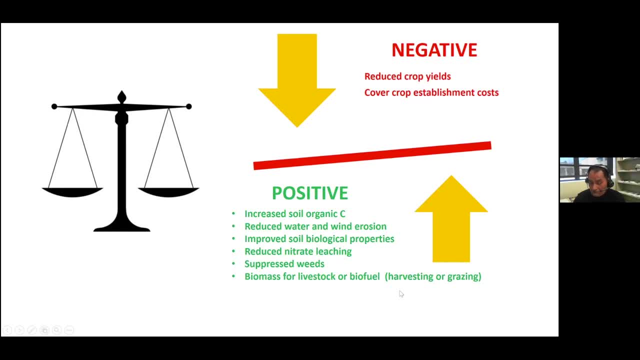 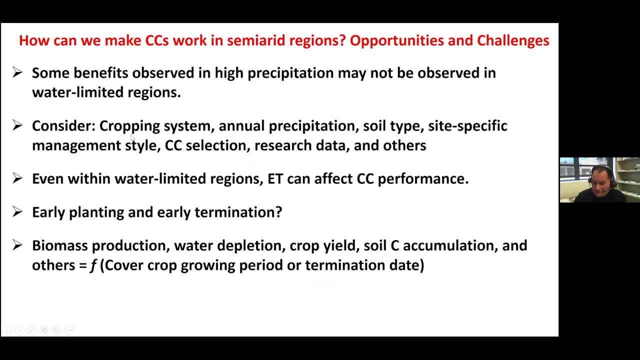 we have not seen, in short, large negative effects of harvesting of grazing cover crop has not reduced the benefits of cover crops in most cases. Well, if you are planning to, you know planting cover crops, we need to think about the cropping system, the precipitation you 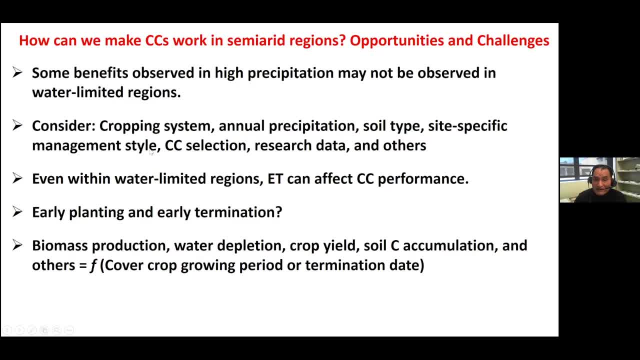 get in your region soil type and the management style, because that could dictate the cover crop performance And then obviously follow the research data collected from the region. So I'm going to stop here, Thank you. I mean ET is one of the main determinants, right? I mean probably cover crops can work. 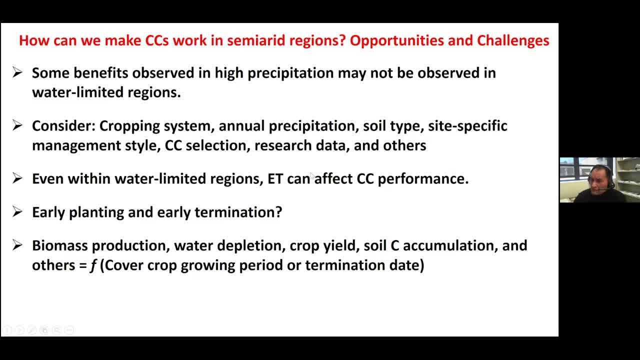 better, Not probably. I've seen cases work better in northern Great Plains because you know it's different than ET. But what about in southern Great Plains? I mean ET is higher, Then under the same amount of rain you are not going to probably get the same. 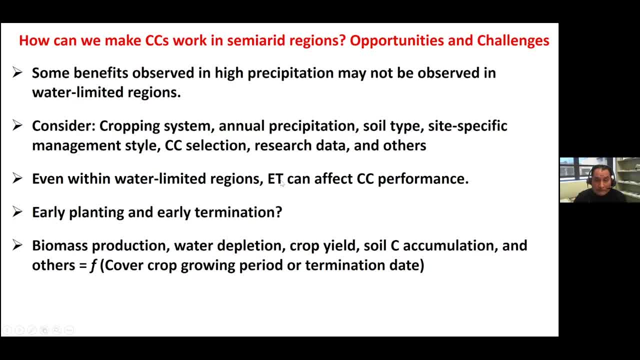 amount of biomass from cover crops in southern and northern Great Plains. What about early planting and early termination? This is something that needs to be done. It needs to be looked at more in detail. And then, obviously, this: you know, determination date, and that dictates the amount of biomass production, Obviously, what it uses in yields. 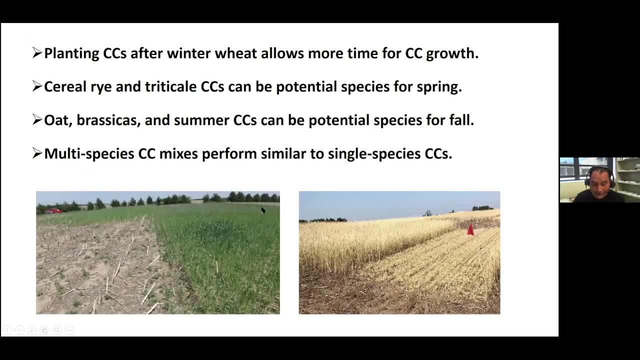 and carbon. I think this is my last slide From you know I worked in western Kansas for many years and we have some experiments in western Nebraska and I see that there is an opportunity there after I mean some Okay. 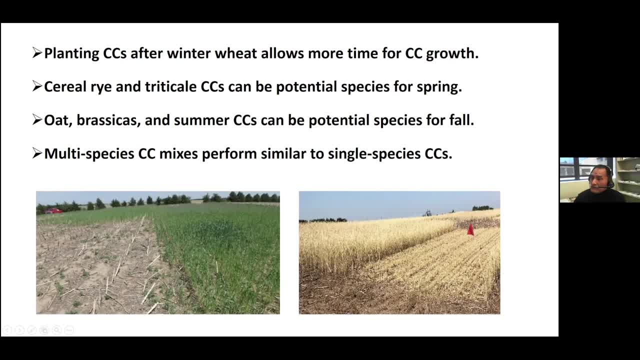 Okay, Farmers are already doing this. I mean planting cover crops after wheat, because we have more time right Growing degree days after wheat they're gonna put some cover crop, some summer cover crops, right Cereal rye- in a triticale. 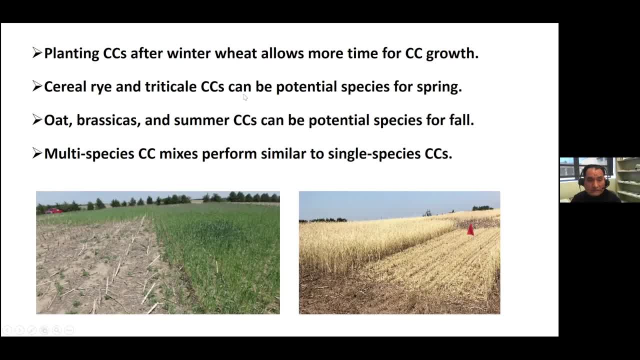 based on the work that we did in Garden City and other places in Western Kansas, I mean, can be potential species for the spring. They produce a lot of biomass, but be careful: If you produce a lot of biomass then we may not have enough water. 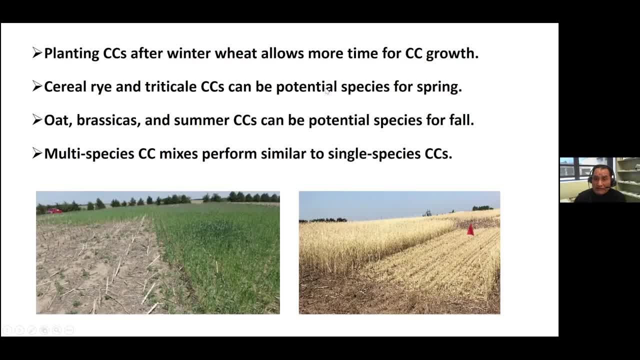 for the subsequent crop right. What about terminating a bit early right? Oat brassicas and some other summer crops can be considered for fall, because if you plant this in July or early August then you can harvest before the end of the year. 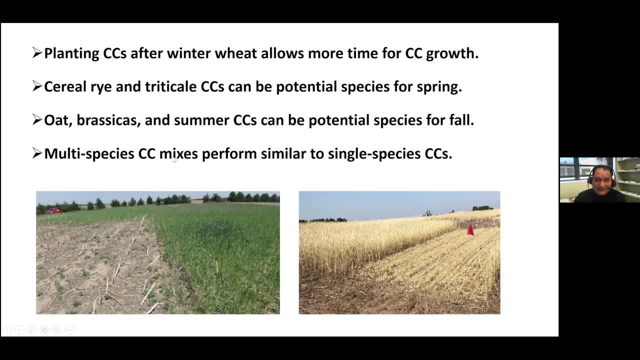 and then you're gonna get a good amount of biomass- Depends again on the year and the rain. And this one, the mixes, You know mixes from what we have seen, from what we have observed is that they do not outperform single species. 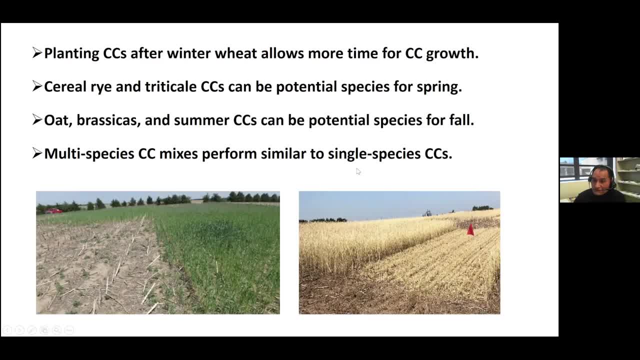 especially the high performing single species. In some cases, those high performing single species can outperform mixes, like rye, for example, right. So, in short, mixes seem to be similar to single species in terms of all the services we discussed about. 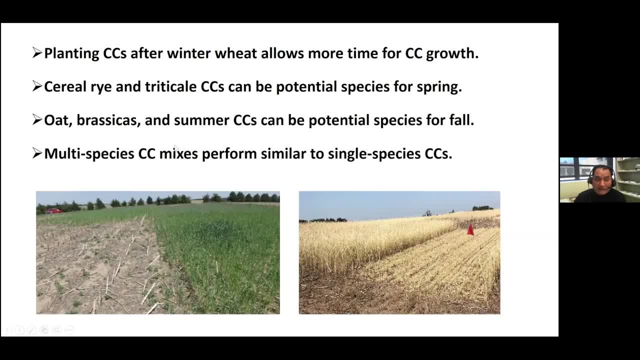 But remember that mixes- right, You need, probably, you're gonna, You need, probably, you're gonna- the cost is going to be higher on their mixes than single species, right? I'm talking about the seed cost, Something to keep in mind. Well, I think that's all what I have. 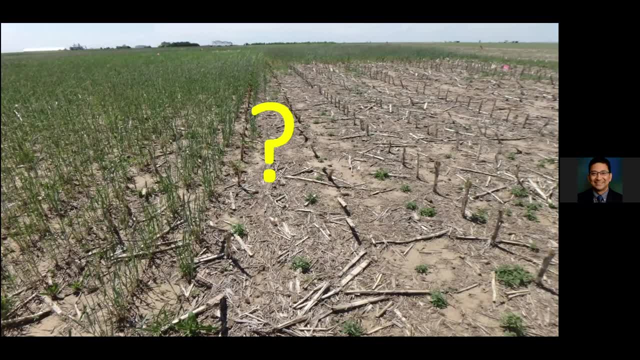 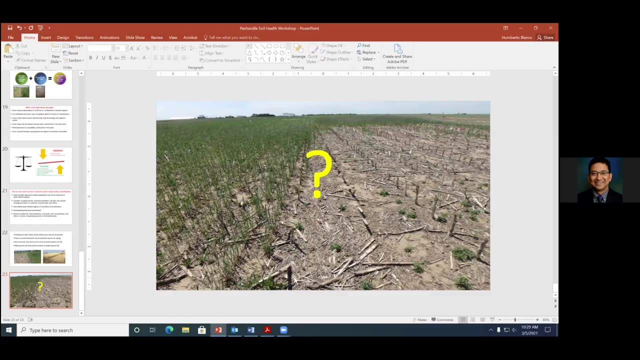 Thank you, Dr Blankos. There are a few questions here in the chat. I'm gonna try to have you address most of them First, pretty brief questions. In your HPAL study, was it corn for grain or silage? I think it was for grain. Wow, I don't think. 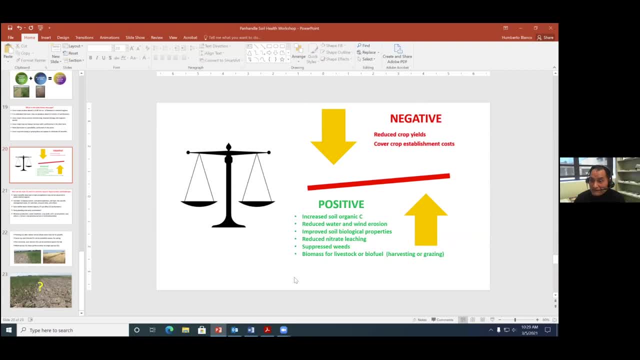 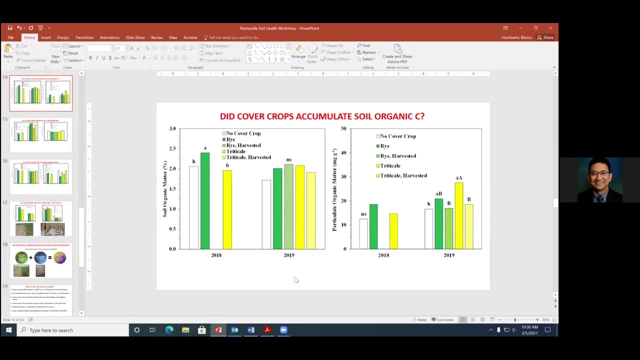 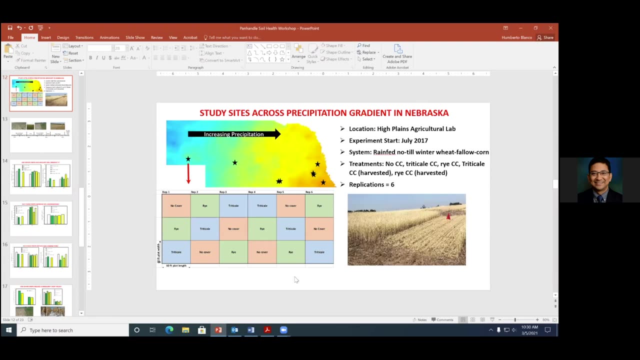 Cody is attending, right, I mean, he has been managing that experiment. So, yeah, 90%, sure it's grain. Okay, One more question before we go to the species question: What's the difference between organic matter and particulate organic matter, and how do they affect the? 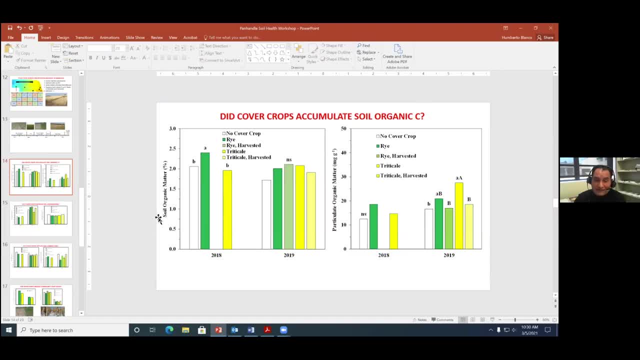 soil, health Good. The organic matter, as you hear, that is on the left. here is the total organic matter content And on the right is the fraction right Fraction. I mean this is the live vial, or what we call fresh organic matter. I mean that which changes, tends to change quicker. 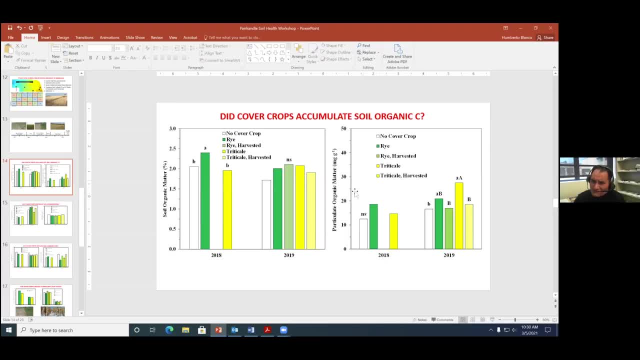 than total. So both of them, I mean this, the particulate organic matter could be more sensitive to management and then obviously, maybe a stronger indicator of soil health changes compared to total organic matter content. Okay, Thank you, And one more last question. I'm going to combine two questions here. One is: 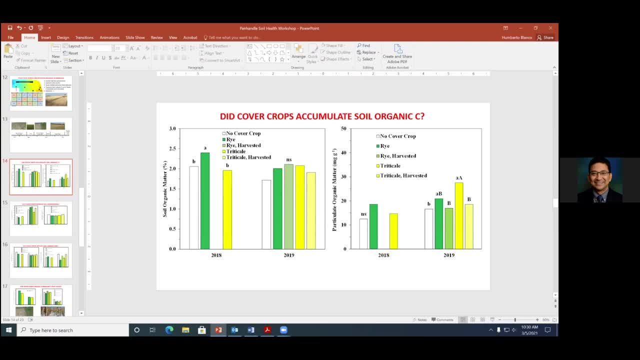 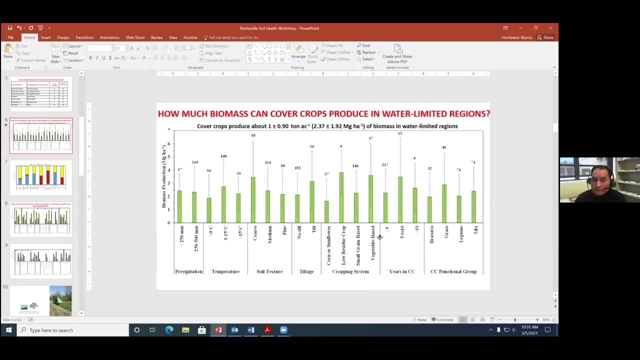 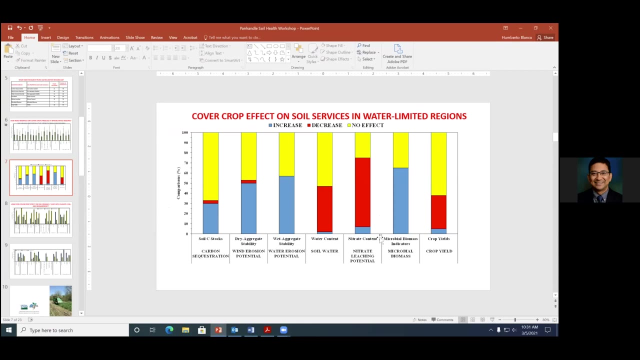 in that first few slides where you presented the effect of cover crops on different parameters, what kind of cover crop or species were used, especially in the water use category? Excellent, Excellent, A good number. I mean we are going to have enough time here to. 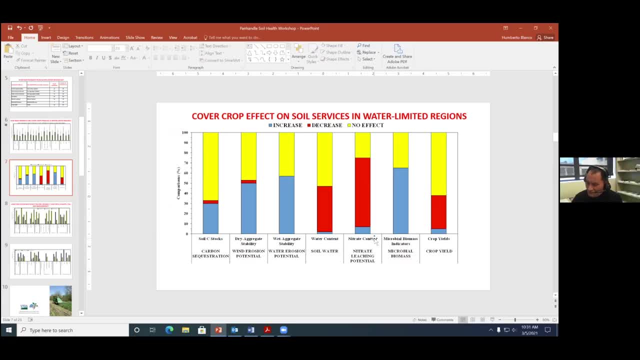 put a table, but rye is one of them. We have triticale, some sorghum sudangrass, but most the leading ones, yeah, those three. We have some pea, field pea, Austrian pea. But if I were to recommend which? 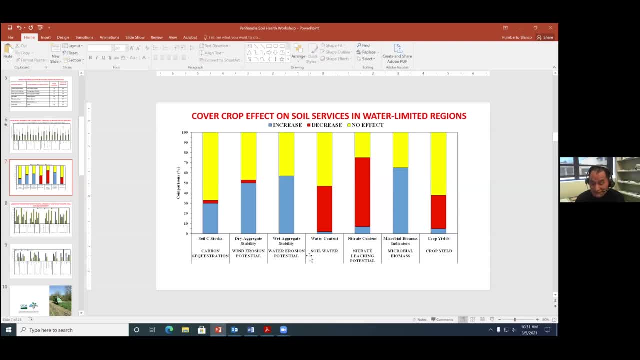 cover crop species should I use? well, immediately, probably, obviously depends on the goal, right on the goal, but the sorghum sudangrass, you know, triticale rye, would be good options and those were used in most studies. Okay, And one final question is probably: 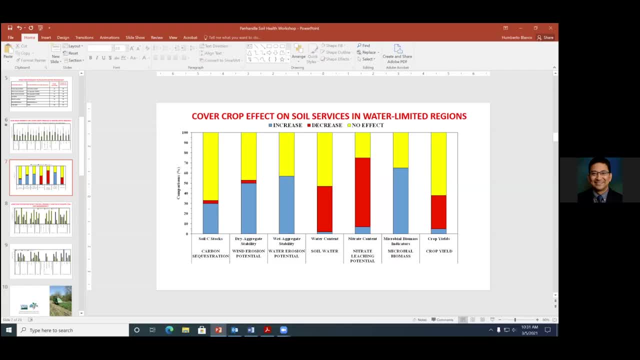 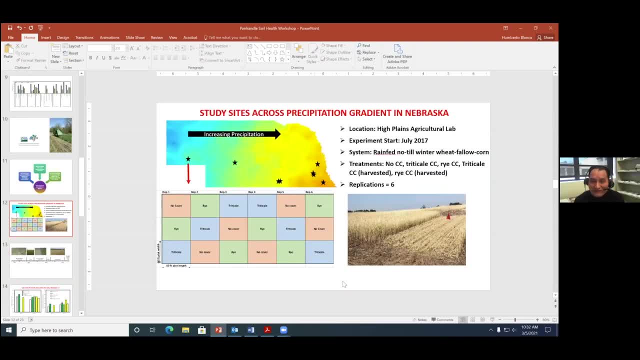 Oh yeah, Thanks for that idea. I'm working on a proposal actually. Yep, Yeah, Excellent. I mean, we're just, you know, getting started with this. They've started harvesting, but what about mixes? Even though, you know, literature seems to indicate that there are no differences. Well,